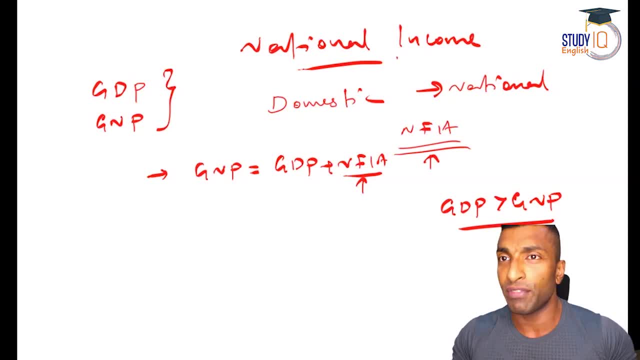 negative. So that's how we have done that. So the point that I have discussed is: if you need to convert any domestic concept to national, like you need to convert NDP to NNP, what do you need to do? Second letter change. So if you have NDP, what do you need to do? NDP plus NFIA? 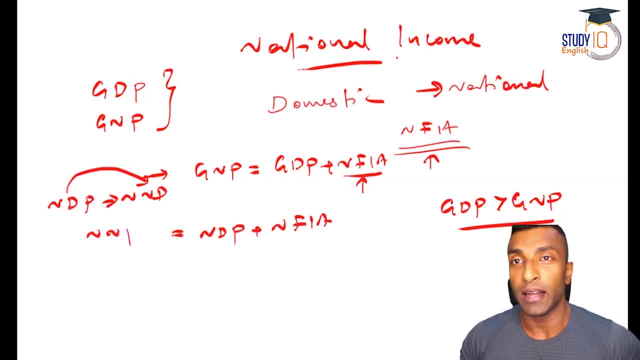 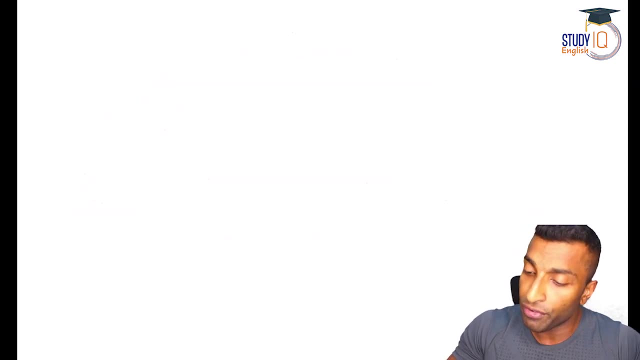 you will be getting NNP. So when you need to change the second letter D to N, this is what you need to do: NFIA. We have also discussed the concept of gross and net, So how to get net from gross. Here we have gross versus net right. So like we have GDP and I want to get NDP, So here. 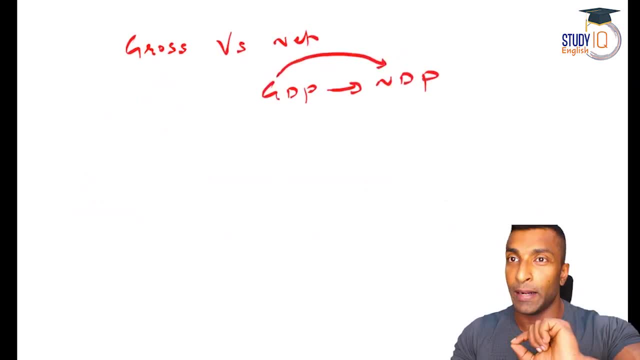 I want to change the first letter gross to net. So what I need to do here I need to subtract the depreciation. So if I have the GDP minus depreciation I will be getting NDP. So if I need to change the first letter, depreciation, If I need 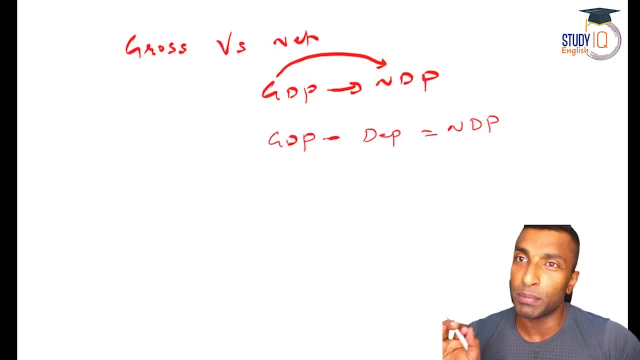 to change the second letter, NFIA. I hope this two concept is going to be very clear to all of you and there is no need to have any confusion with respect to this. Similarly, if I need to convert NNP, GNP to NNP, what has changed First letter? what I need to do- GNP minus depreciation- you will. 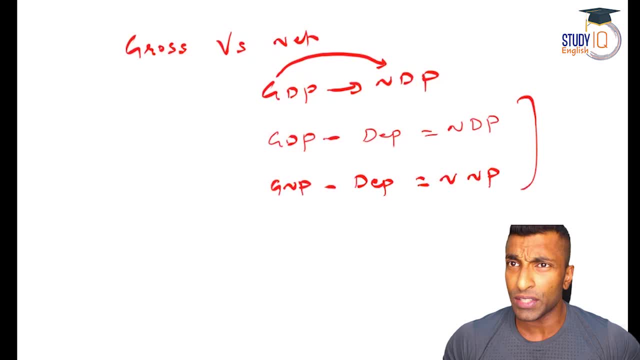 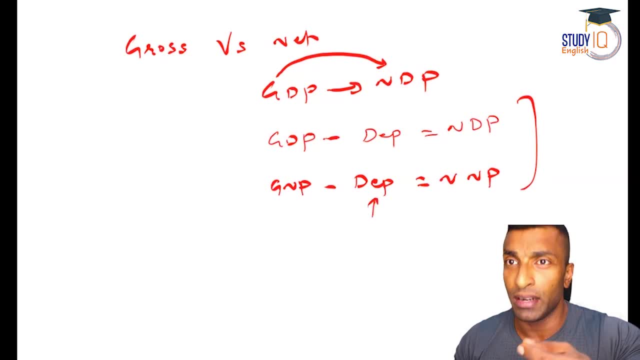 even though NNP is not a depreciation. Why you are not calculating NNP is better because you are considering the depreciation. Why we are not calculating that NDP? mainly because to calculate the depreciation there is no uniform method or uniform measure. So that is a reason why. 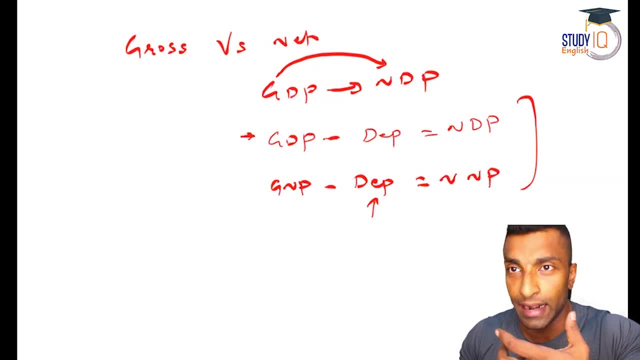 for the purpose of making things easier and because of the international best practice, we always go for gross, because that is very easy to calculate. Measurement of depreciation is difficult and then there is no uniform method in which you can do that. So what we will be doing in this session is- I've told you in the beginning itself, there are 16 concepts related to national income. 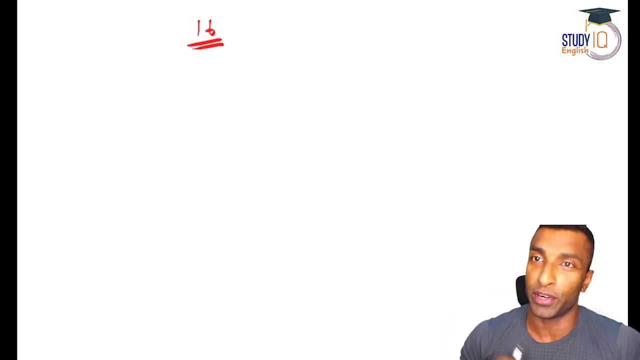 It is nothing but the permutation combination of four important concepts, out of which we have discussed two: Gross versus net, we have done. Domestic versus national, we have done- And I hope all of you understood that We have to discuss only about NFIA and depreciation- That two thing is done. 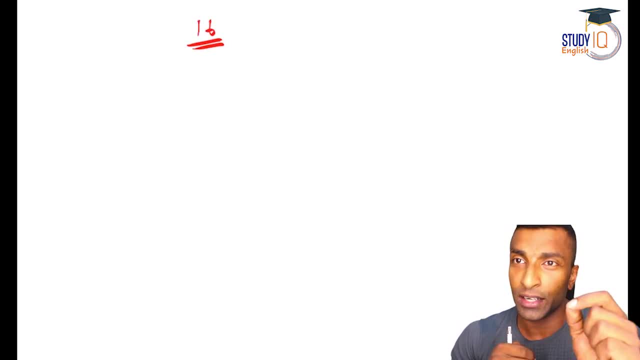 Now, here I'll be discussing about factor cost versus market price. Let's understand that, And then we'll discuss about current versus constant prices. So, once we understood these four important concepts, the permutation combination is going to give you the 16 concepts, and then I'll discuss exactly what is national income. 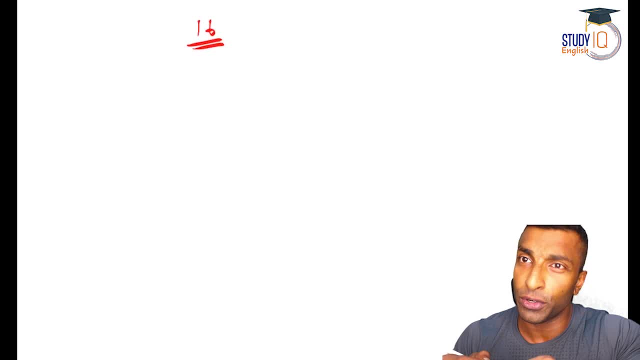 Okay, so let's go with the factor cost versus market price, just like what we have done before. Here also, there is some additions, There is some subtraction which is going to give you the other. Okay, so let's I'll just give the heading factor cost versus market price. 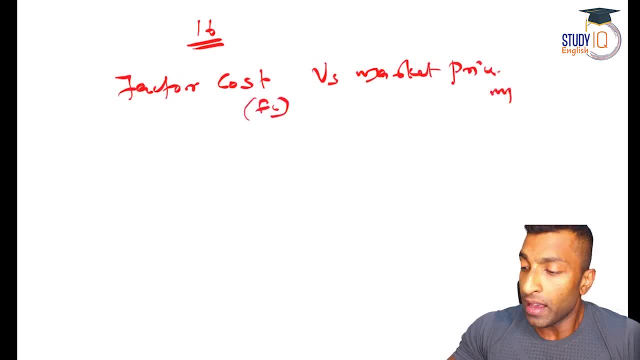 Okay, so you will be writing it as FC and MP. So this is what we need to discuss now. So, guys, what is factor cost? It is nothing but the cost incurred on factors. So it's like: what are the factors? factor inputs, land, labor, capital, entrepreneurship. 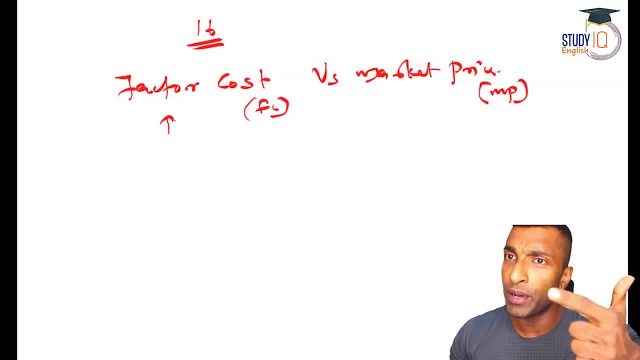 So what are the costs Which is incurred on that land? it is rent, labor, it is wages or salaries, capital, it is the interest, entrepreneurship, it is a profit. So that's what actually comes in this part. Okay, so we will not be considering profit here. 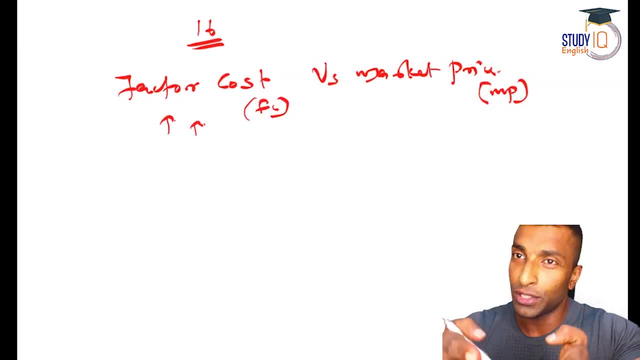 You see, if you have studied in CSAT factor cost or the cost price and market price, the difference between that is actually profit. But here you don't want to have that confusion. Whenever I talk about profit it is part of entrepreneurship which is actually added. 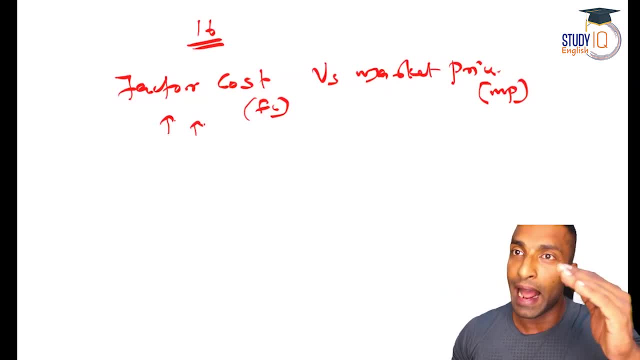 In the factor cost itself, because factor inputs land, labor, capital, entrepreneurship. So profit is actually coming within factor cost. So no need to have confusion with respect to profit, which is also a kind of value addition, which is actually part of factor cost. 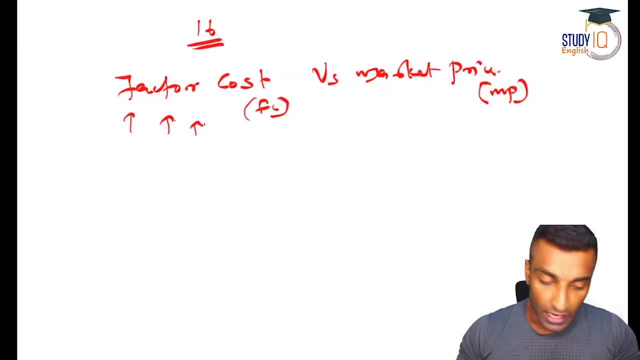 So what is the difference between factor cost and market price? If you ask me, it is nothing but like the taxes. Okay, so market price equal to the factor cost plus net indirect tax. I'll explain what is net indirect Guys. it's just like this, only I'll just expand it further. 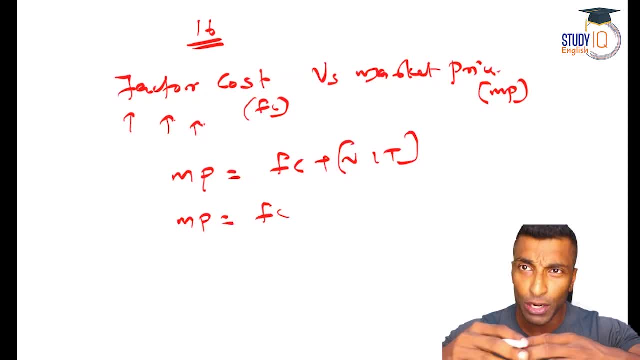 Market price equal to factor cost. That means the actual cost of production, which include the profit, plus taxes, which is imposed on government, and indirect tax, because direct tax is imposed on income, wealth, etc. So here I'm talking about indirect tax, which is imposed on goods and services. 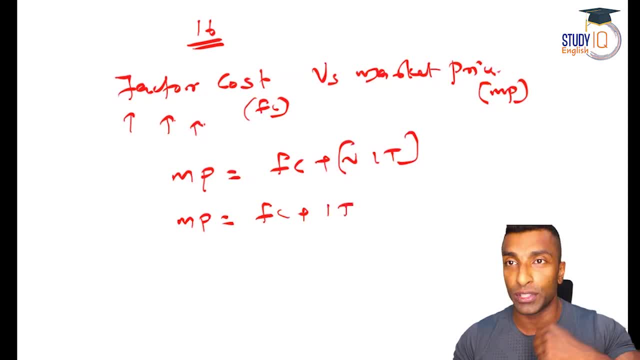 So factor cost plus taxes imposed on goods and services. And guys, for some situation, for some products government Have to give some subsidies, some essential products like that. So that need to be excluded. So I'm excluding the subsidies. Okay, so this is what you know. net indirect tax. net indirect tax means the difference between indirect tax and subsidy. 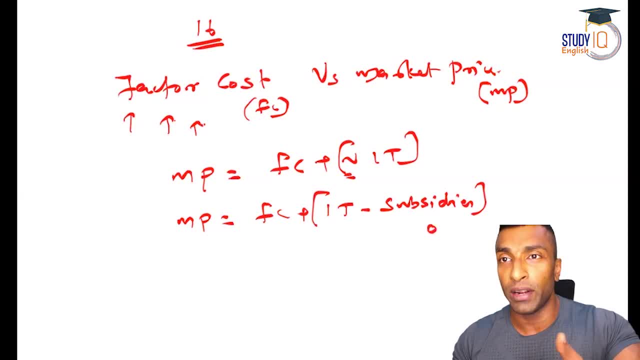 So sometimes subsidies are zero. Sometimes subsidy will be given, So that is the reason why I've taken it as net indirect tax. Some item subsidy won't be there, So you'll just put it as zero. Sometimes subsidies there, So you need to. 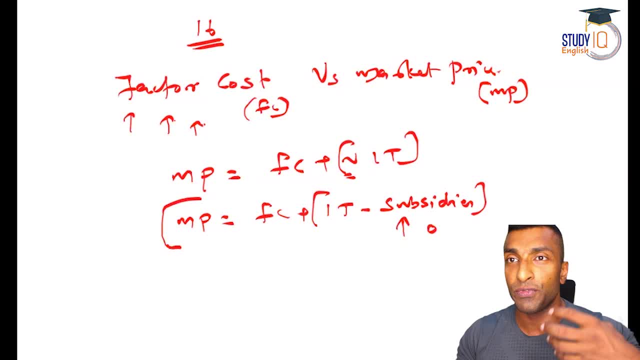 Exclude that. So what is market price? Market prices: factor cost plus net indirect tax. Now I hope this part is very clear. So GDP market price If I need what I need to do: GDP factor cost Plus net indirect tax. 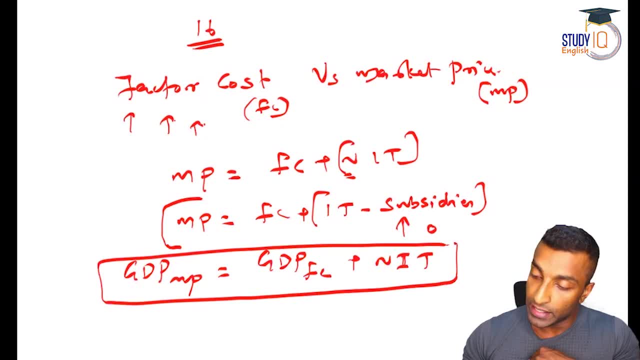 Okay, so GDP market price equal to GDP factor cost plus net indirect tax. So since I've written It as net indirect tax, I don't want to write it separately like this. So some books you will see: GDP factor cost plus indirect tax, minus subsidies. 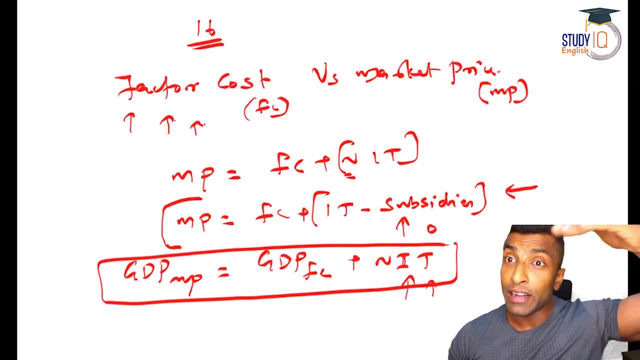 Instead I'm just writing it as net indirect tax, like net factor income from abroad. What was that? income earned by foreigners from India minus income earned by Indians from abroad. Just like that tax minus subsidy here. So net will be taking that difference and will be added to this. 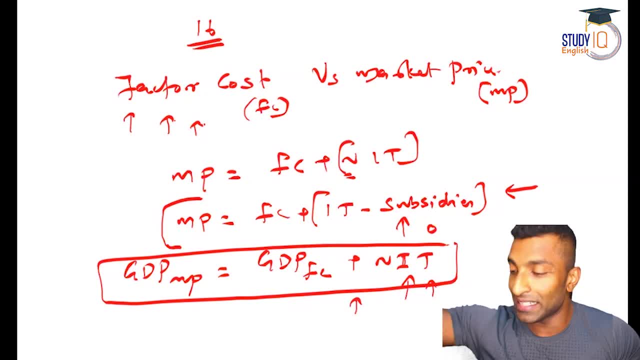 Obviously it is Unlike the previous case. this is going to be positive, because you're not going to give more subsidy than the tax. Okay, so there it was negative NFIA, but that's not going to be the case here, anyway. 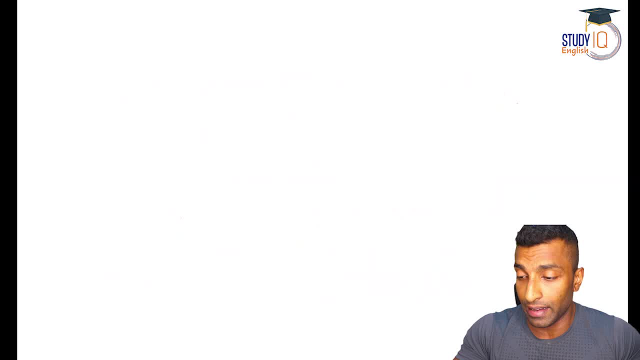 So I hope this is very clear. What about, like NDP, net domestic product at market price? What do you need to do? NDP at factor cost plus net indirect tax. So how to get market price, factor cost plus net indirect tax, But which one is easy to get from the market. 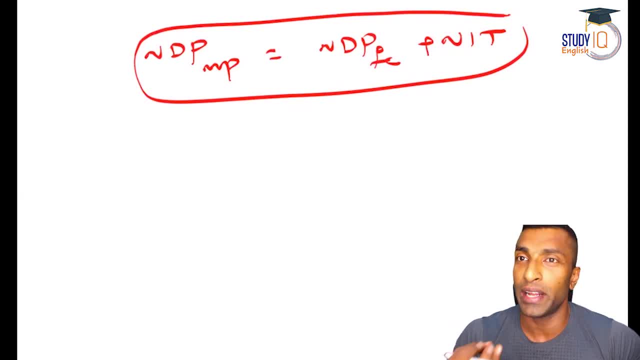 You will be getting the market price because transactions and everything is actually happening at the market price. So you collect it at market price and exclude the net indirect tax, You can get the factor cost also. So for calculation purpose you can do it in any way. 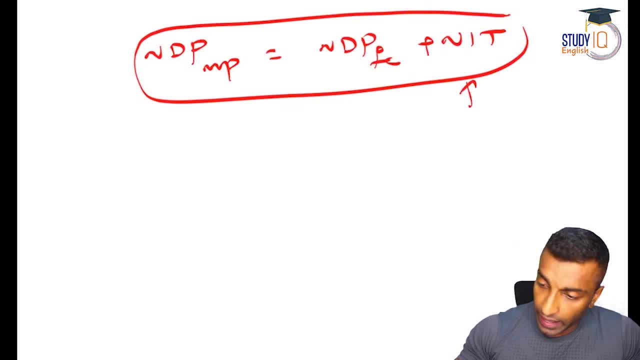 I hope this is very, very clear. So why only indirect tax? I'm taking That logic is very clear, because the direct tax is imposed on income, wealth, etc. Right, So I don't want to. I don't want to discuss about that anyway at this juncture. 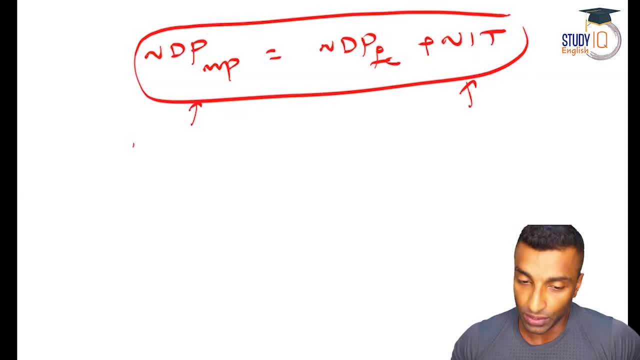 So it won't. It is not going to affect the value of goods and services, So direct taxes are actually imposed on the income. that I have anyway discussed in the chapter of the module on taxation. So direct tax is imposed on income, wealth and activities, on individual right or the forms. 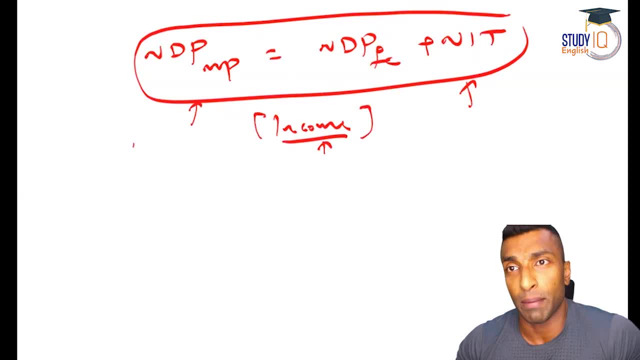 So if you see, there is income tax for the individuals and for the companies, there is corporate income tax. So, and for wealth? wealth tax is there, House tax is there. So these are not going to affect here. That is the reason why we are taking the indirect tax. 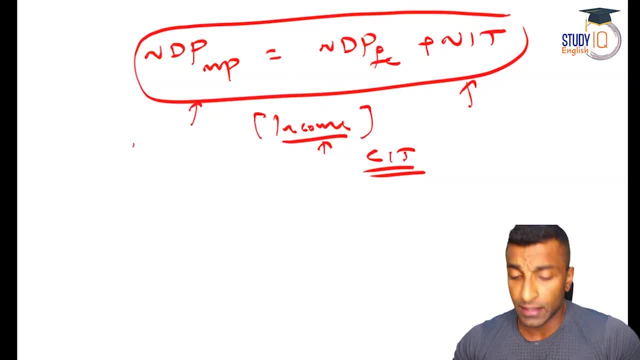 So that part is very clear, Right. What is subsidy? Subsidies are the government grants to forms or individual. OK, so taxes are imposed on the forms and you have to take the burden. You have to pay that, just like that. 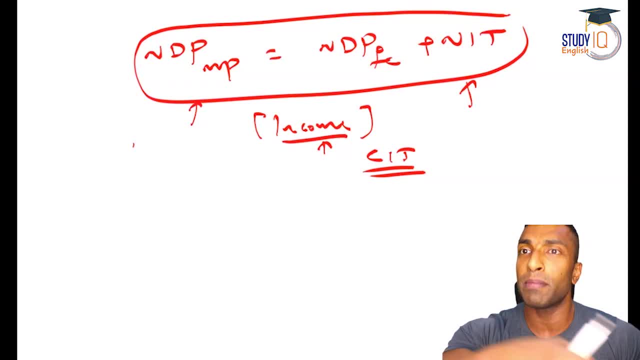 Subsidies are given to the firms but the individuals we will get benefit out of it. So this part Part is very clear. Net indirect tax means indirect tax minus subsidy. So that is about factor cost versus market price. Now, guys, which one is used for actual transaction market price? 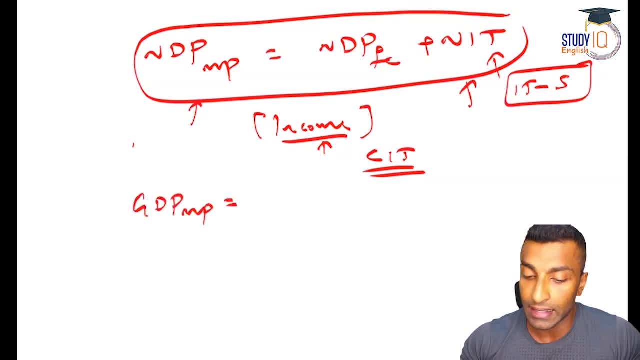 So which one is easy to get? GDP at market price is easy to get because this is used for direct transaction. Then what is GDP FC factor cost? This is for the measurement And guys, till 2015.. Till 2015.. For the purpose of calculation of GDP. 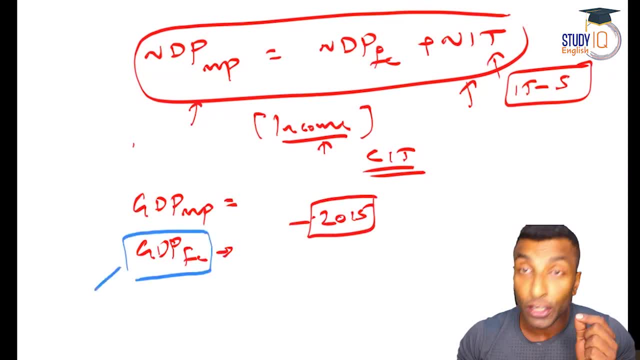 GDP. we were using GDP factor cost till 2015.. And there is a change in national income methodology from 2015,. I'll be discussing towards the end of this module. And now we have shifted to GDP market price, because it is very easy to calculate market price, because the transactions are done. 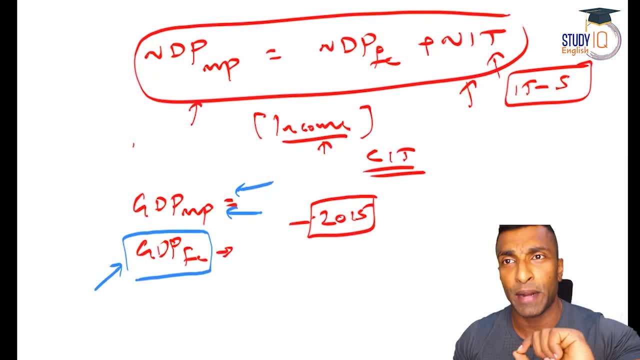 at the market price And secondly, this is the international best practices and also for that reason GDP market price is used to calculate the GDP from 2015 onwards. But there is a problem in that there can be a lot of manipulations, which can be done right If the government want to show. 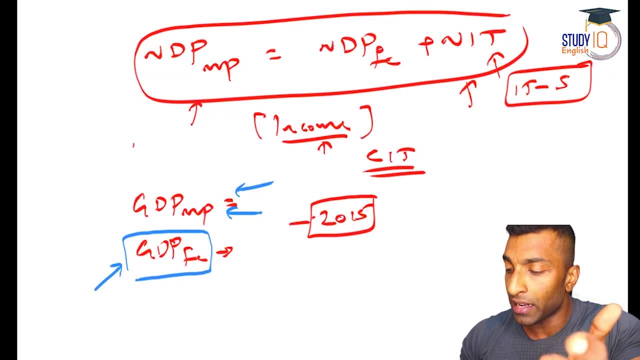 a higher GDP. what the government can do is government can increase the market price. How the government can increase the market price? you just simply increase the tax. If you simply increase the tax, what can happen? Obviously, GDP at market price will also increase. So if the 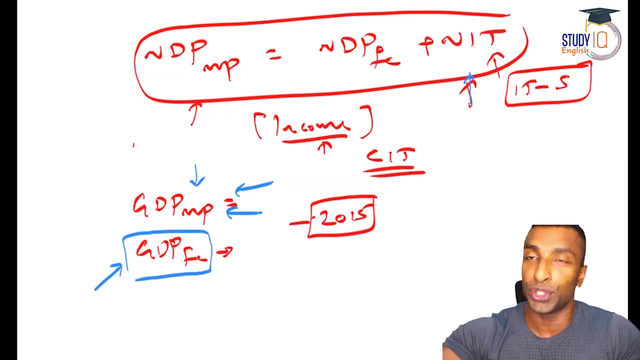 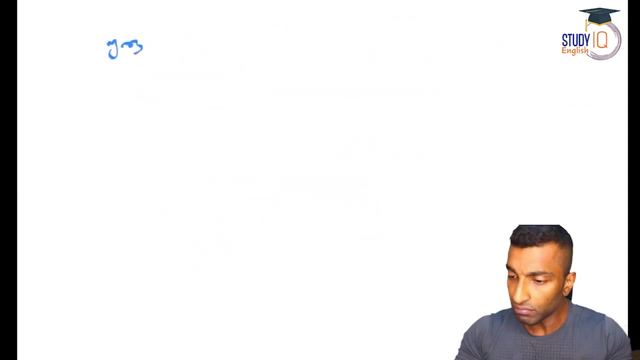 government want to portray image, or government want to show that GDP have increased? government can simply increase the tax even though the production is less, even though production have come down, but still just. but I'll just show you an example. with this, things will be very clear. But let's talk about two years. 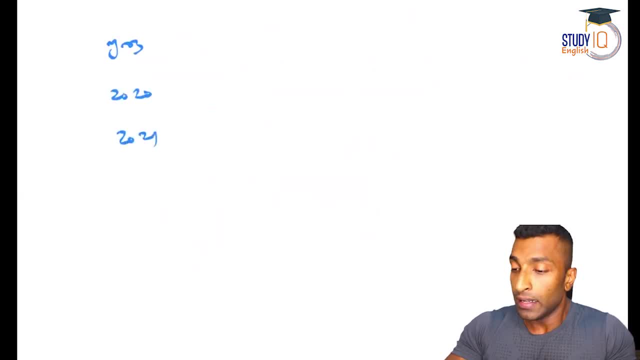 let's say, 2020.. And then 2021.. So let's see, I have a company, manufacturing company which produced this pen. okay, so the production of pen and I have produced around 100 pens and in 2021, also 100 pens. So, in terms of actual production, is there any increase? No increase. 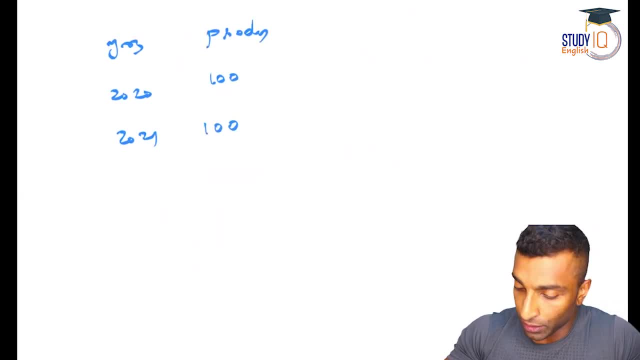 it is the same right. So let's see the factor cost. Factor cost means the value addition that factor inputs. the value addition will come from four factor inputs: land, labor, capital, entrepreneurship. income will come only through value addition. value addition can come. 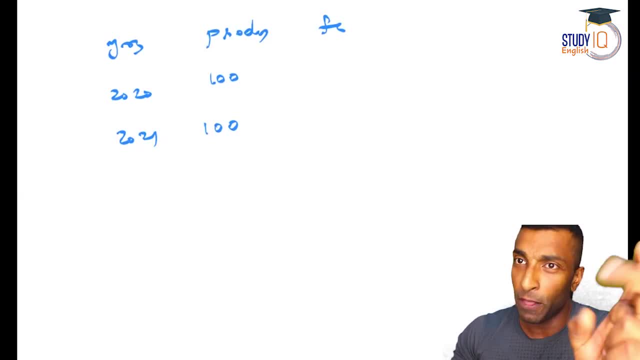 only through factor inputs And these are in the form of rent wages, interest on the capital. So in the form of rent wages, interest on the capital, and then the value addition will come only through value addition, capital and the profit. Okay, so that is very clear. So, factor cost, let's say nine, nine, it's. 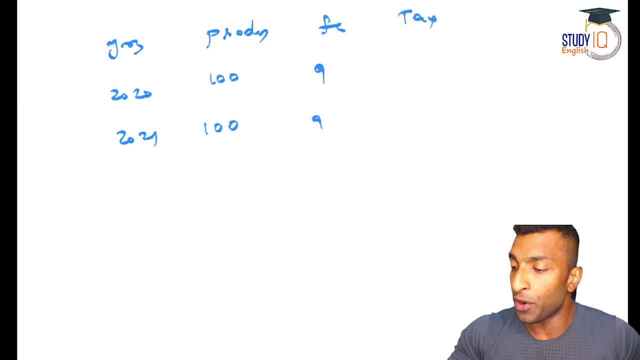 the same. Now, let's say, tax is one rupee and the government increased to two rupee next year. So what will happen to market price? Just ignore the subsidy here. I'm not talking about subsidy for the pen, Okay, so it's not that essential item or anything. So market price, if you see it is going. 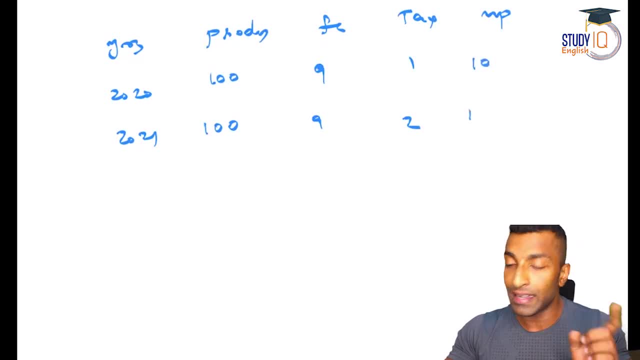 to be nine plus one, that is 10 rupee, and nine plus two, that is 11 rupees. the market price have increased. Remember. production remains the same, the cost of the pen stays the same and also the same factor cost remain the same. tax have increased because of that market price. have 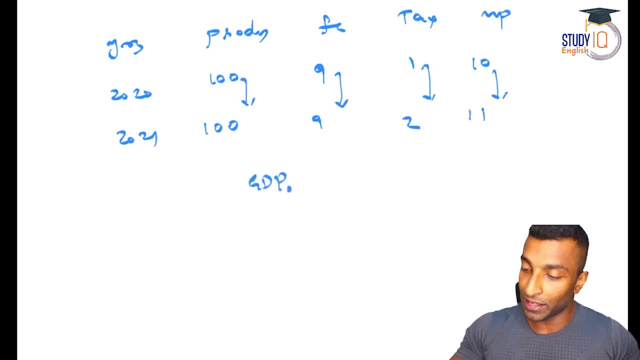 increased. Now let's calculate GDP at factor cost and GDP at market price in both years. So GDP at factor cost: 100 into 9, that is going to be 900.. Next year also, it is the same factor cost if you calculate 900, but if you calculate it on market price it's going to be 1000, and then it is. 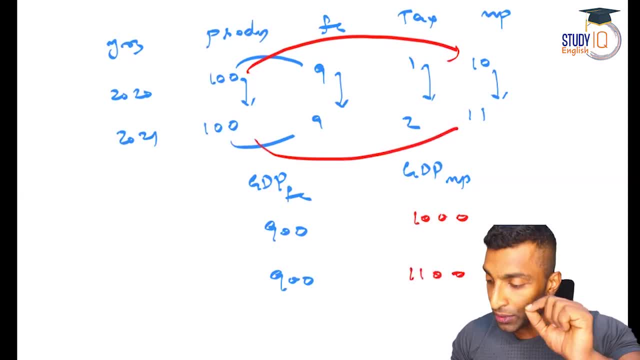 going to be 1100.. So if you look at factor cost, is there any change in GDP? No change. there is no growth because actual production have not increased. but if you look at the market price, is there any change? There is a 10% change, right. So what you can see is you increase the tax by 10%, that's. 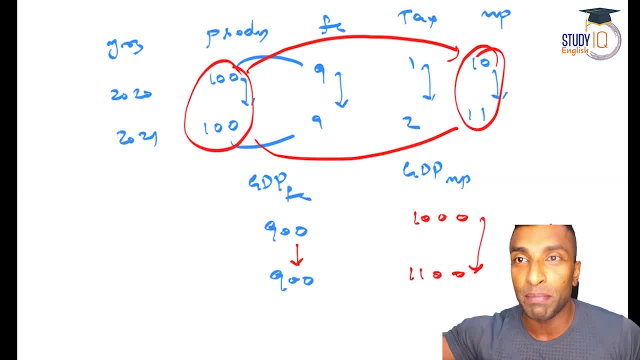 exactly what you have done: 10 to 11.. So what has happened with the GDP at market price? you have increased. you are able to show that 10% increase in GDP. So what the government can do is simply by increasing the tax, you can actually show that the GDP have increased. This is actually the drawback. 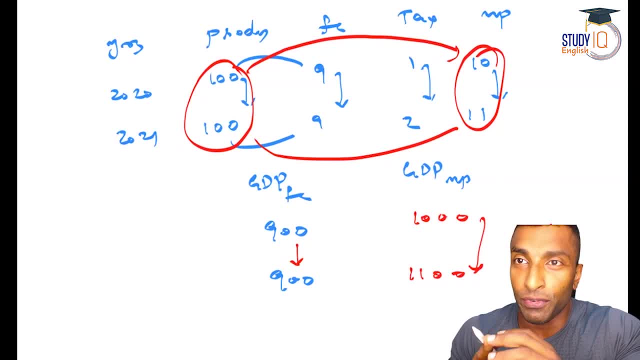 So, guys, which one is better? in terms of calculation of GDP, Factor, cost is better because this will show the growth only if there is an actual growth in terms of production. On the other hand, market price- if you calculate it can show a higher GDP- depends on the price. 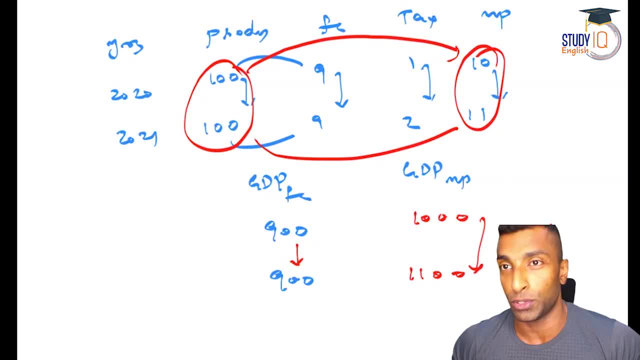 increase, which may be due to the increase in taxes also. So that point need to be very clear and there is a very important concept that has to be there in your mind. So this is one of the drawback, in case, if you are getting a mains question, you need to be in a position to 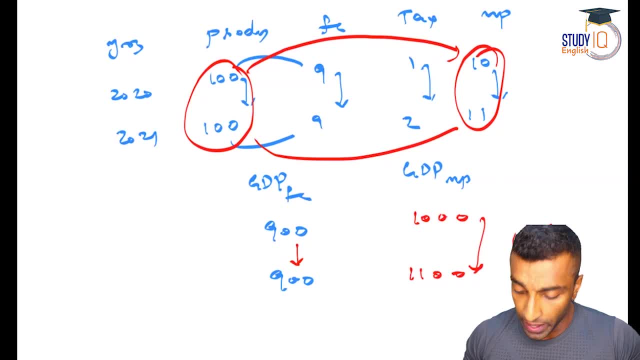 explain this exactly in this way, But still, obviously the question is why market price we are going for. It is the international best practices. transactions are done at the market price and easy to get market price when you get it from the market and everything. So for that purpose- calculation wise also, it is very 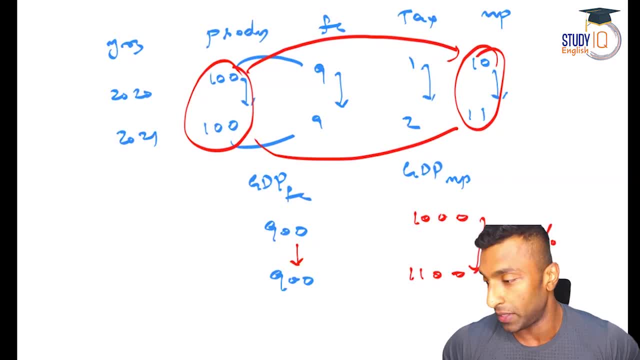 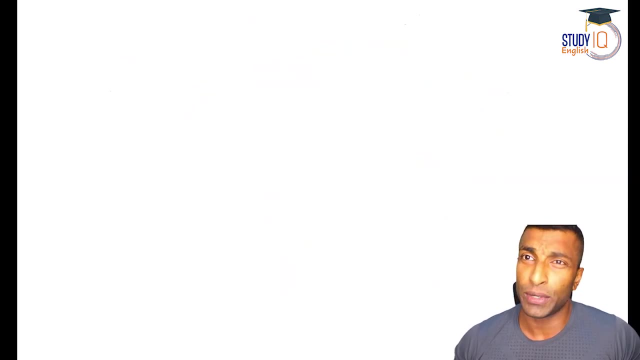 simple. That way, you will go for market price. So if you need to substantiate, these are the ways in which you need to substantiate. If you need to tell the drawback of it, you can even show this and you can explain it. I hope this is very, very clear. Most of the students have confusion, but 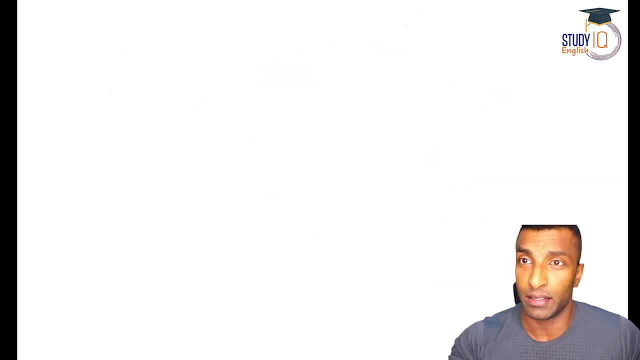 when I am explaining with the numbers, it has to be very clear. Now, next is the current prices versus constant prices. What is the difference between this? I will just write it down: current price versus constant price. So, guys, current price is the prevailing price. Let's. 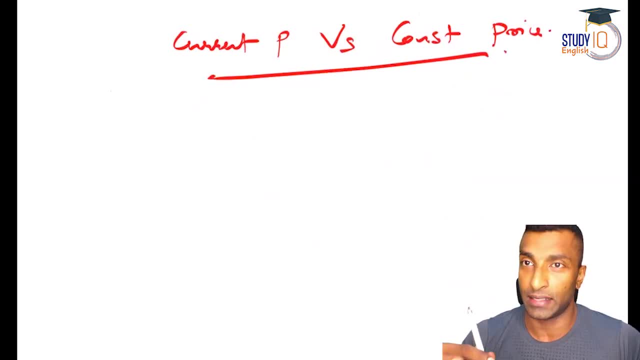 say I'm talking about this pen. If it is 10,000, this is a current price in which I can buy from the market. Constant price is the price of this pen on a particular base year. So I'll be fixing a base year. Let's say now, currently we are using 2011-12 as the base year. There is a proposal. 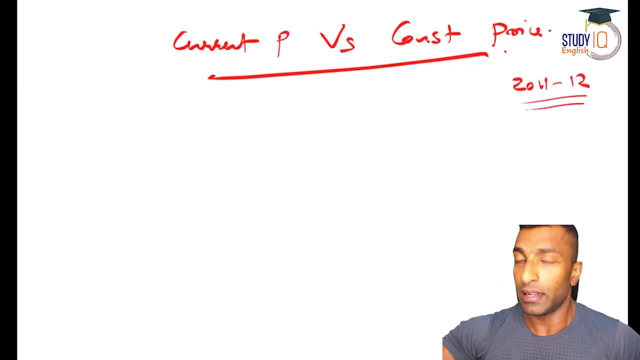 which is going on: 2022-2021.. The base year has to be changed to 2020-2021 because we need the latest year as much as possible. That is one of the criteria for taking the base year. So there is a proposal which is going on and we'll be discussing about all those things in the coming. 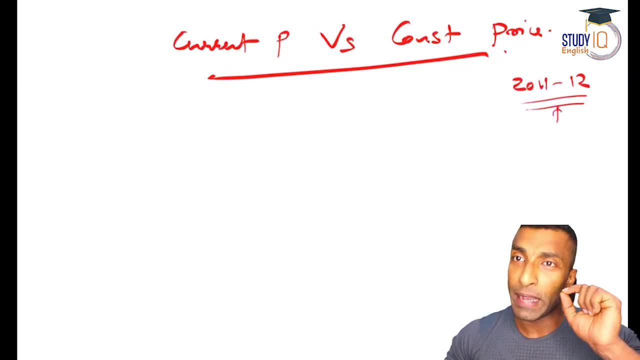 session. So as of now, 2011-12,. so what is the base year 2011-12?? What was the price of this pen in the base year? Let's say if it is 5,000 or 6,000, that is going to be your constant price. So the price. 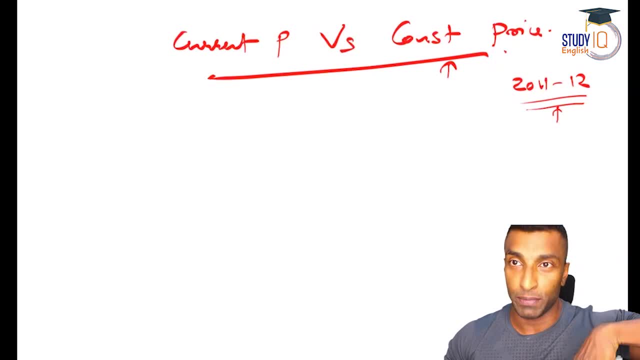 of the item in the base year is going to be the constant price. Now, let's say 2020-21, the pen cost around 10,000.. So if you change this as the base year, the next year onwards when you calculate the, 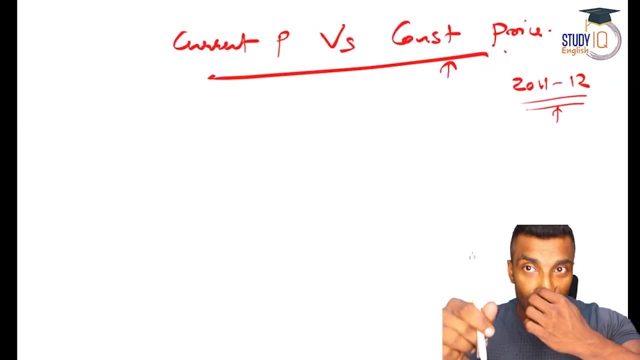 constant price. it is going to be 10,000.. So the price of that item on the base year that year, what was the price? That will become the constant price and it won't change till you change the base year. But the current price keep on changing. Why Inflation, This pen? 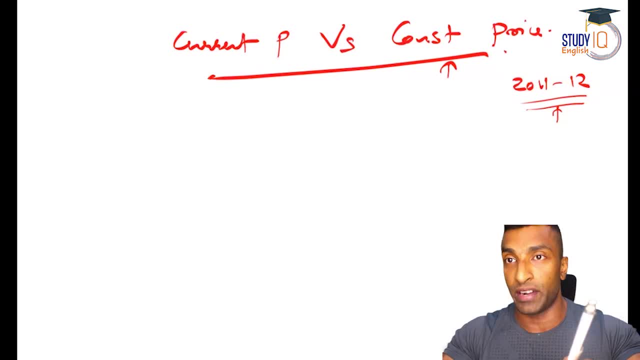 is 10,000 now. Next year, if there is a 7% inflation, it is going to be 10,700.. Next year there is another 7% inflation, that is going to be 11,500.. Like that, it keeps on changing. Current price, keep on. 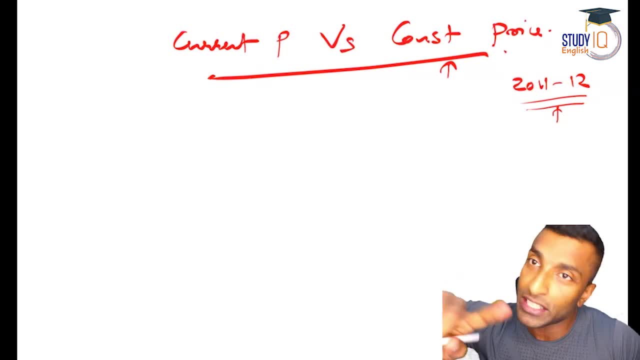 changing based on inflation. Constant price will change only if there is a change or a revision in the base price. So from 2011-12 onwards- till now, the price remain the same because that's the base year. Okay, Now which one is? 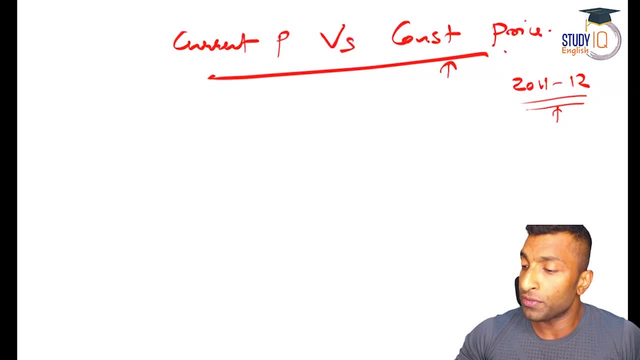 used to calculate Guys, for calculation of GDP. constant price is actually what we are using, But otherwise, normally to explain or express something in terms of percentage, like when we discuss about fiscal deficit etc- then we will talk about the current price. So I'll just show. 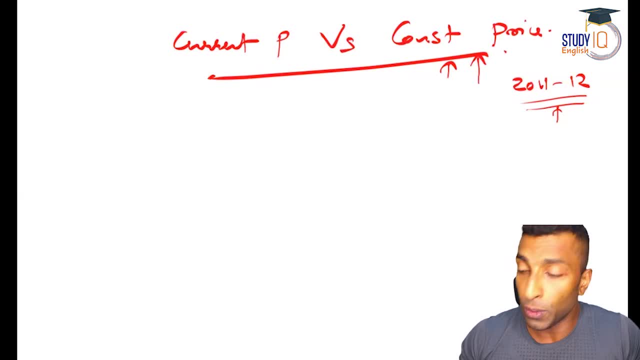 you this one and why we are taking constant price also, The difference. I hope it is clear it is inflation, So we can calculate that based on GDP deflator, which is again an index number which is used to measure inflation. I can explain what is GDP deflator with example also, and I'll 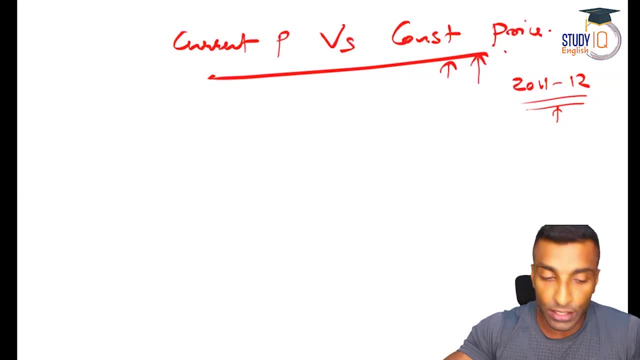 show you how it can be calculated as well. So again, I'll just draw a table. Let's talk about three years. Can we go with 2011-12, since it is a base year? I'll start with that because I can. 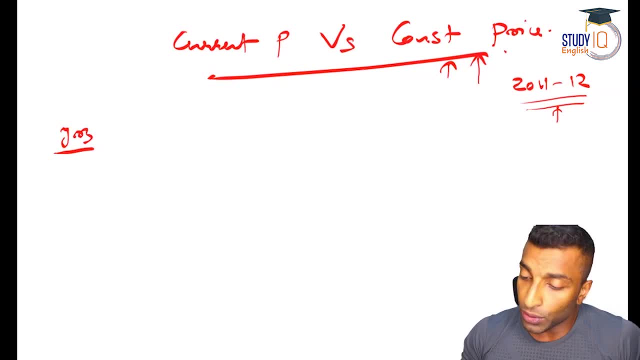 show you how base year price is calculated. So let's talk about 2011-12.. Since that is a base year, I'm starting with that And then 2000.. 2012-13,, 2013-14.. Now let's talk about the production of the same pen. So let's say: 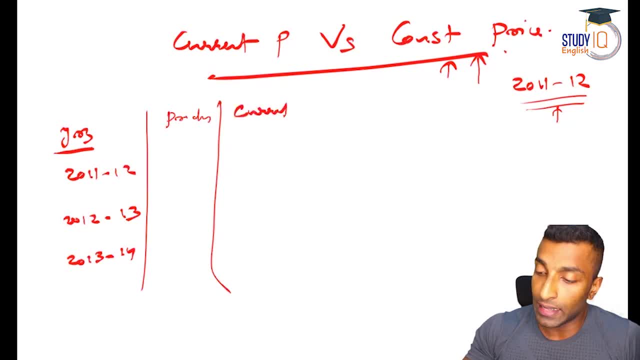 production. And then I'll talk about the current price. That means the current price in which I can buy it. And let's talk about the base year price. Guys here, what is the base year? 2011-12 was the base year, So the price in the current price of 2011-12 was going to be the constant price. 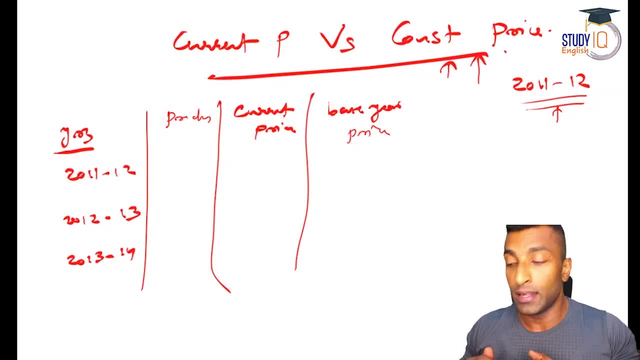 next year onwards, It is the same. It won't change. So now let me talk about production. let's say 100.. And the current price in 2011-12 was, let's say, 10 rupee for the pen. Current price of that year is going to be the. 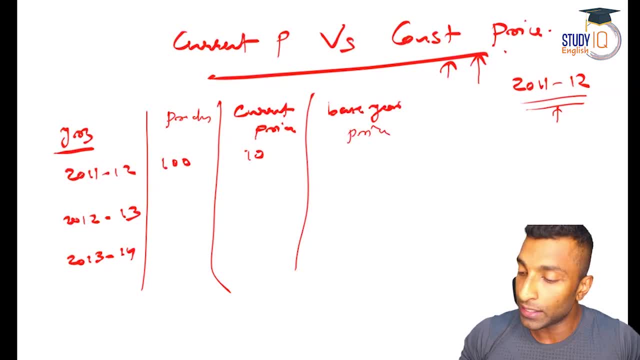 constant price or the base year price. So that is going to be 10.. And now it won't change The constant price. now it is not going to change, But the current price will change based on inflation. So let's say, next year prices increased to 15 due to inflation. But here you won't find any. 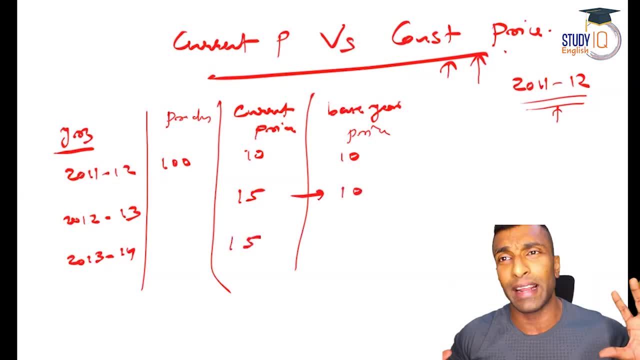 change. It will be 10.. Next year there is no inflation or anything. Just take it as 15 itself. I'm just taking random examples to explain different scenarios which are possible. So here it is going to be 10 again. It won't change. And let's add production also. Let's say production there. 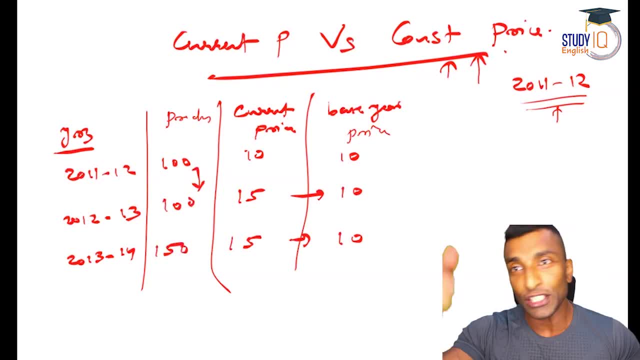 is no change And let's say, production, there is some change. So, because I can discuss different situations, Okay. So that is the reason why I'm taking these numbers. And now let's calculate GDP at current and GDP at constant. So GDP at current and GDP at constant, So GDP at. 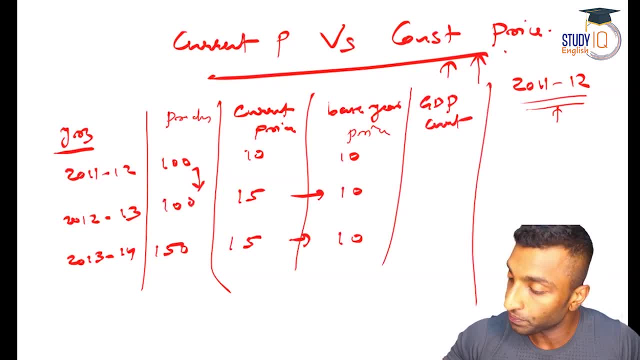 current that is going to be 1000. Then here 1500. And here 2250.. And now GDP at constant, if you see 1000. And then here 1000. And here it is going to be 1500.. Now listen very carefully. 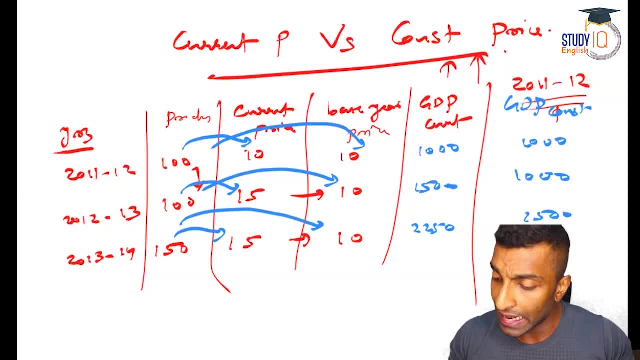 guys. First here, if you see, is there any change in production? No change in production. So is there any change in GDP? If you see GDP at current price, I can see change, But if I see GDP at constant price, I can't see change. Why current price? GDP have changed. 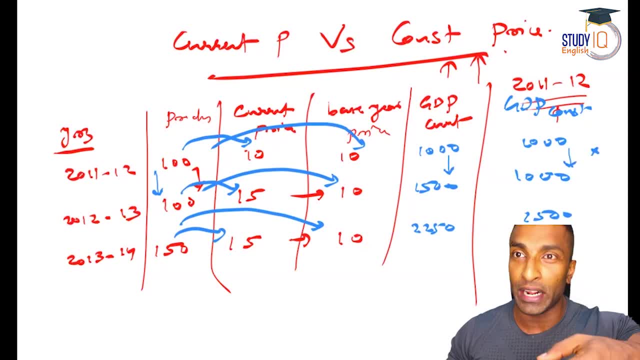 Because of inflation. Though there is no increase in production- actual production- I can see a change in GDP because of inflation. So my point here is that current GDP is going to increase, But if I see it at current price, I'm going to see change. So if you see GDP, 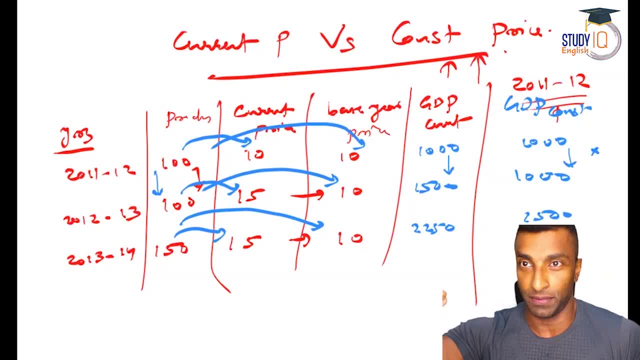 at constant price instead of constant production, I can see that the current GDP is increasing. So you see there is an increase in production. So that means if you look at our current GDP, if you calculate the current prices, it can increase due to inflation, But constant will. 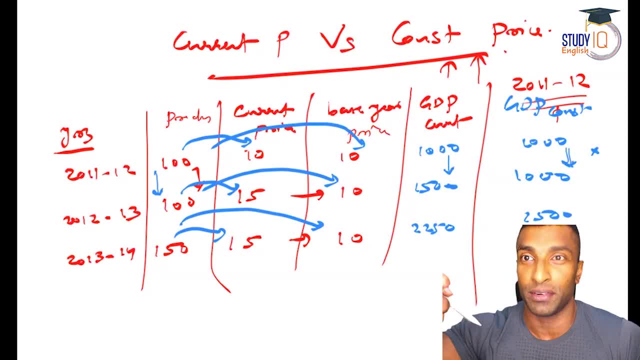 change only if there is an actual change in production. Otherwise it won't change. Now again, if you see the next one, there is an increase in production, Right? So here I can see increase in production. Here also I can see increase in production. So here. 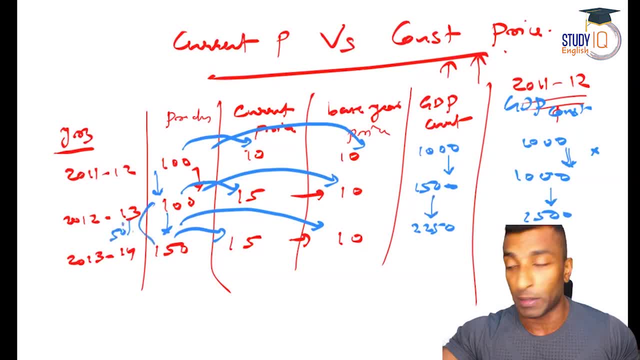 what percent increases there? 50%, 100% to 150%–50%. So here also I can see exactly 50%. So if you calculate at the constant price, whatever percentage change in the production, actual production, exactly the same percentage change you will get when you calculate at the. 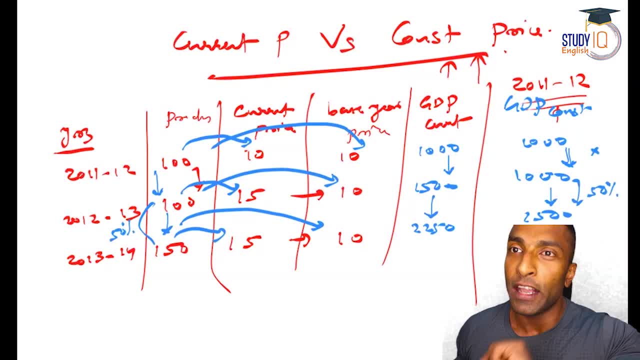 constant price. Now I'll make it very clear. If you calculate GDP at the current price, it will increase either due to actual production increased, like here: actual production increase, no inflation- or due to inflation. So current price GDP may change, either due to inflation. 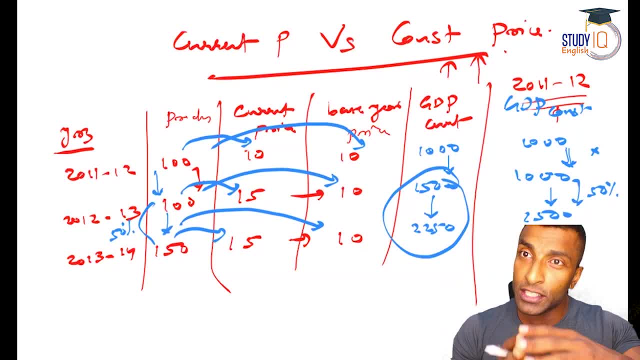 or due to actual change in production. But the constant price will change only if there is an actual change in production. So which one is better? The constant price is better. So that is the reason why we guys it depends on certain prices, right? So it depends on the constant price. 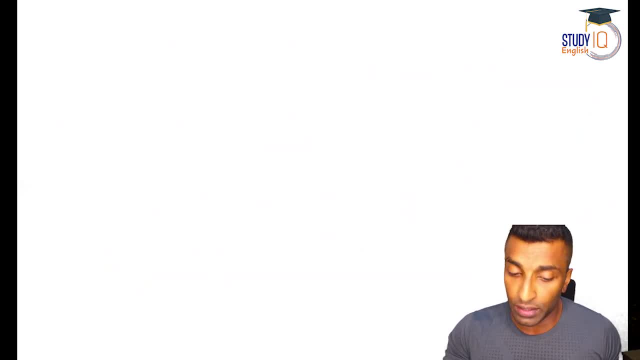 the base year and everything is actually connected. So see, when we normally calculate, we take it as current price, because that is very easy to get from the market right. So, and then you can adjust it with base year And when we discuss about as percentage of GDP or 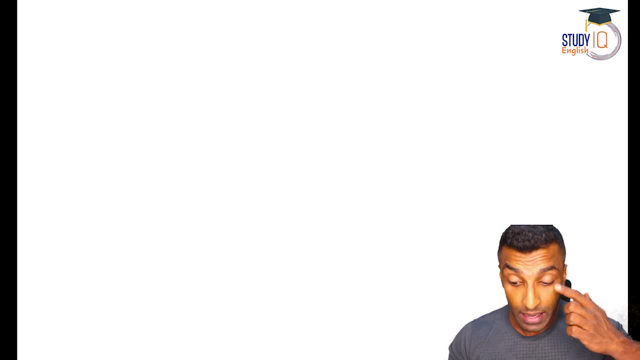 fiscal deficit during that time. also we will talk about market price. But when we calculate the growth that time, we use the constant price. Now what we get from the market, we get the current price, But for the current price we use the constant price. So what we get from the market, 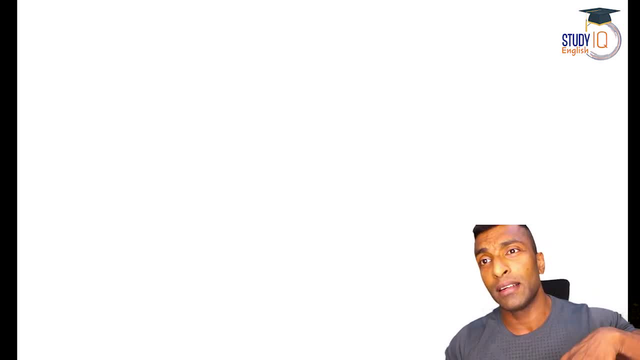 for the calculation. we need constant price. How are we going to get that? Adjust it with inflation. How are we going to adjust it with inflation? There is an index number which used to measure inflation- GDP deflator- So I'll be just talking about that also. Okay, Now, guys. 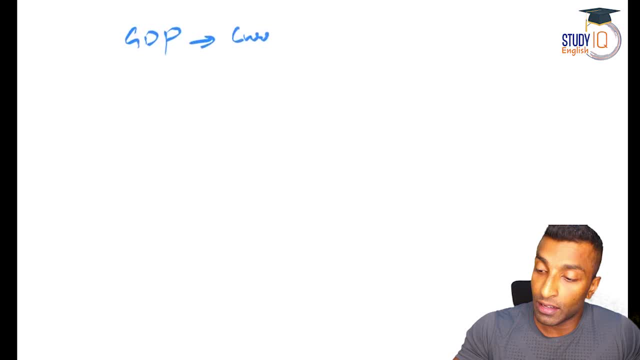 GDP. if you take it current price, this is what Nominal. Current is always nominal Nominal GDP. If you take it constant price, this is the real GDP. Okay, So for making reference, for making comparisons, we use nominal GDP. For the calculation, we use real GDP. That means a: 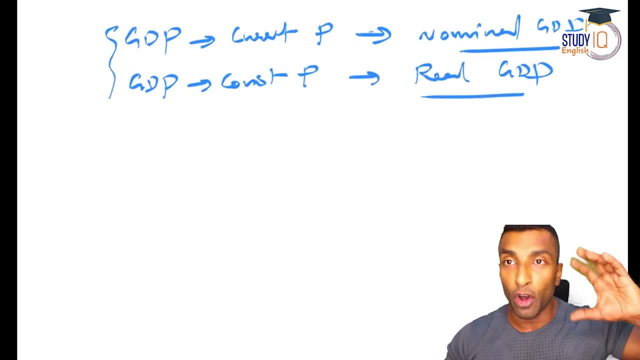 constant price. I hope this is very, very clear. So nominal is always the current price. Real is a constant price. Guys, later I'll be talking about NNP at factor cost. This is your national income. NNP at factor cost- This I can take it constant. 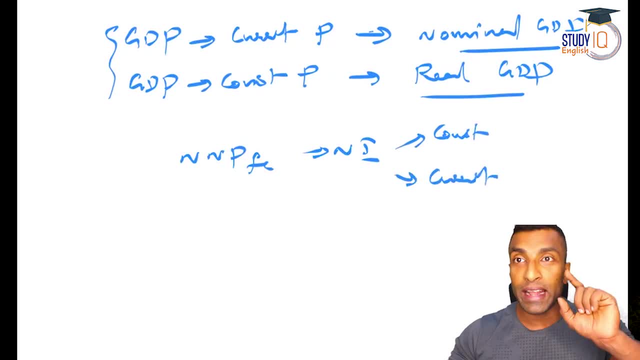 This: I can take it current. So if I take it at constant, this is your real national income. So whatever you take at constant, that's real, And if you take it current, that is your nominal national income. Similarly, I can take NDP at factor cost Here, domestic, So this is your. 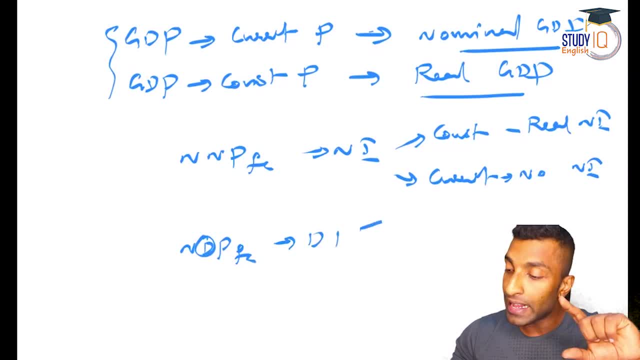 domestic income, NDP at factor cost. Here also I can take a constant price, I can take it current price. So constant price if I take, that is the current. So if I take NDP at factor cost a real domestic income, if I take it at current price that is a nominal domestic income. So I 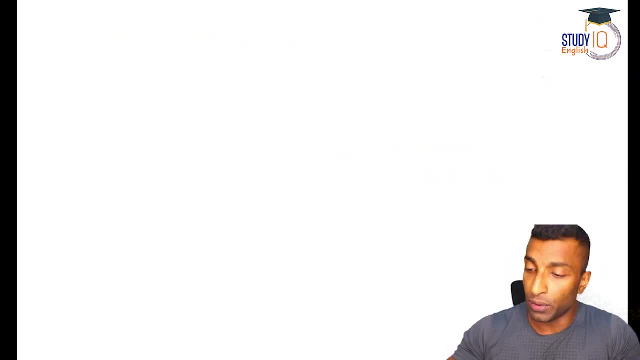 hope this part is very, very clear. So if I need to discuss about: okay, so what we get from the market, we get the nominal GDP means at the current price, what we need, we need the real GDP. What is real GDP? GDP at constant price. I want to get GDP at constant price from GDP. 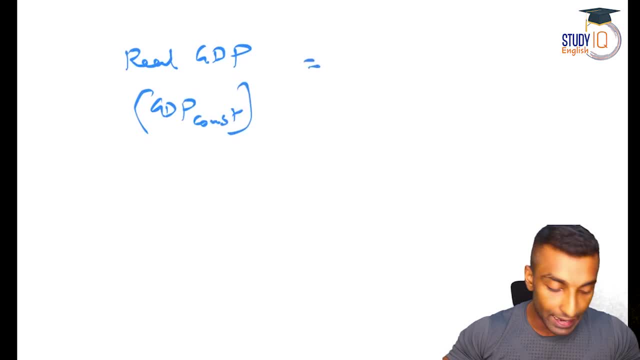 current price GDP. current price is nominal GDP, So how can I get it as like this? So I'll just write it as nominal GDP. I want to get real GDP from nominal GDP. Nominal GDP- in bracket I'll write it as GDP current. So what I get is GDP current divided by GDP deflator. That's the. 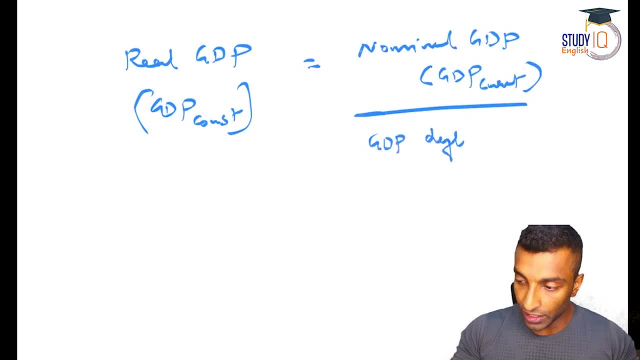 index number I have discussed- GDP deflator, and then multiplied by 100.. So that you'll get it in 30.. Okay so, as I've told you, this is an index number which is used to measure inflation. Okay so it's. 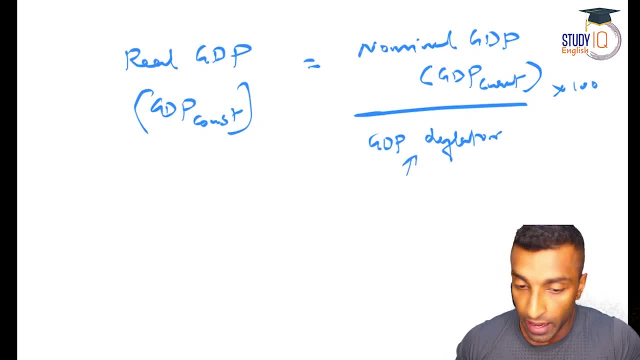 a variable. obviously it's a statistical tool which is actually used to measure inflation. So like price, production, population etc. So it vary. So based on that you can measure. So for GDP deflator you need again a base here and a base value, because if I simply tell the price of 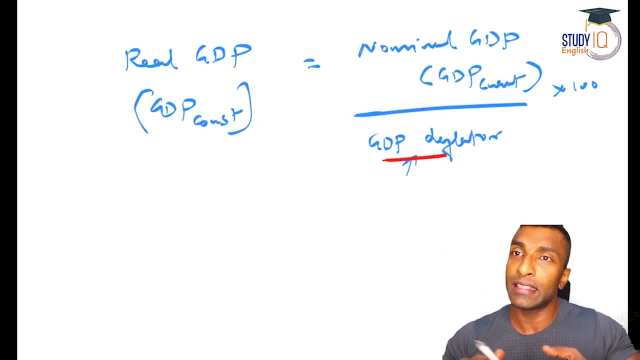 this pen is, let's say, 25 rupees, you won't understand anything. I can say the price is increased, But you won't understand what increased, from where increased, to what extent it has increased. For that what I need, I need a reference value. I need a reference here. Reference value is your base. 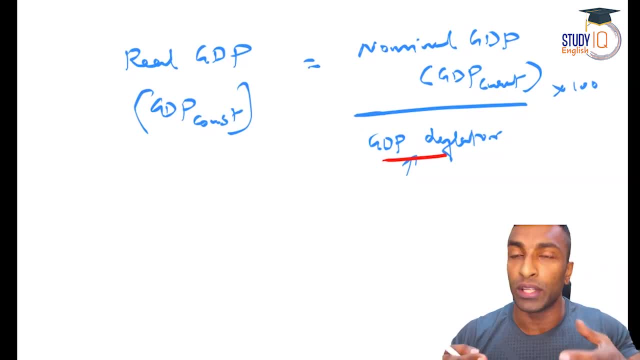 price Reference here is your base here, So I need both. then only I can actually tell to what extent the price of increased or decreased right. So like, if you see WPI, how is it calculated? It is also an index number, So you will be writing like this: WPI, then a colon, and then 2011-12,. 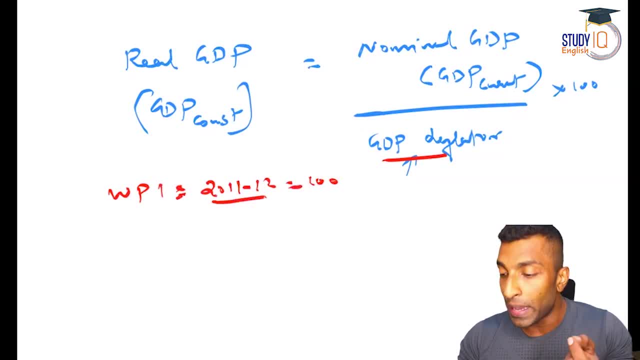 which is the base Here? let's say 100.. So 11-12 is the base here, 100 is the base value, reference value. Now, if I say it, this 100 have increased to 147.. Now 2020, then what does that mean? There is an inflation of 47. 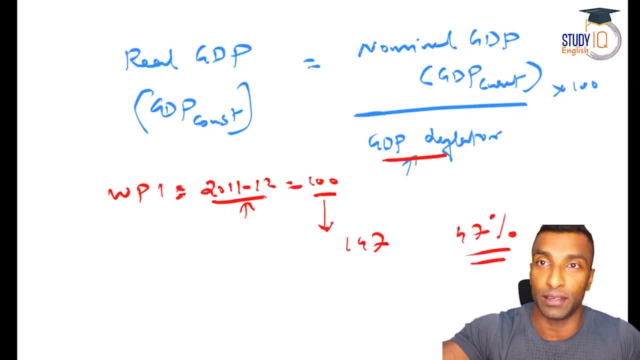 percentage from 2011-12, from the base year. Just like that, you can write: you know this also. CPI also based on your similarly GDP deflator. how will I write? Yeah, we have a deficit of 42.. The deficit of 43 deflator 2011-12,, which is the base year, equal to 100.. 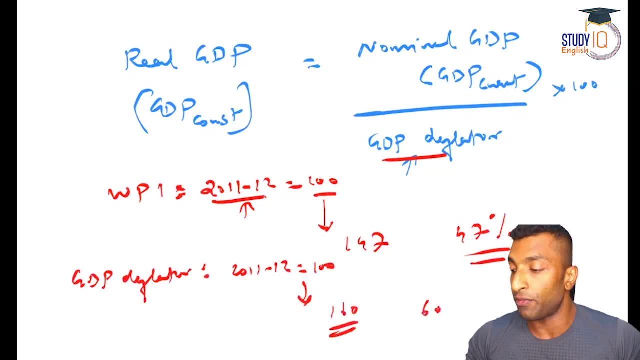 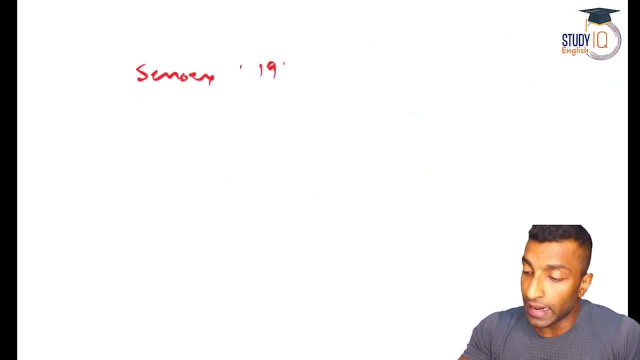 Now, if it become 160, means what That is? a 60% inflation. That's what you need to understand. Same way, if I want to write SENSEX, what is the base year? 1978-79, which was started at 100.. 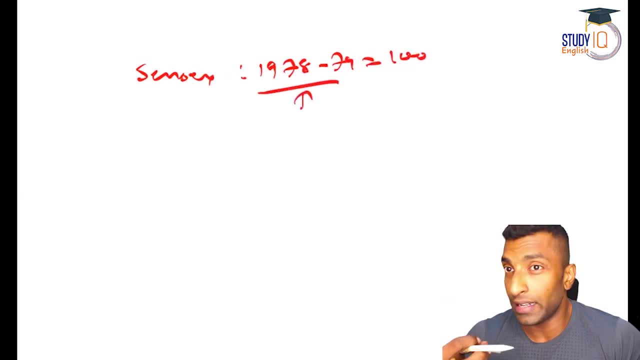 Guys, I have told you the base year need to be earliest as possible. but it is not possible in case of SENSEX, Because now it has grown like 50,000, like this, and I don't know if I have any sense of it. I know it can't be 100. But the EPA will change. Guys, this I have told you: the base year need to be earliest as possible. But it is not possible in case of SENSEX, Because now it has grown like 50,000, like podia. so it is kind of strange. 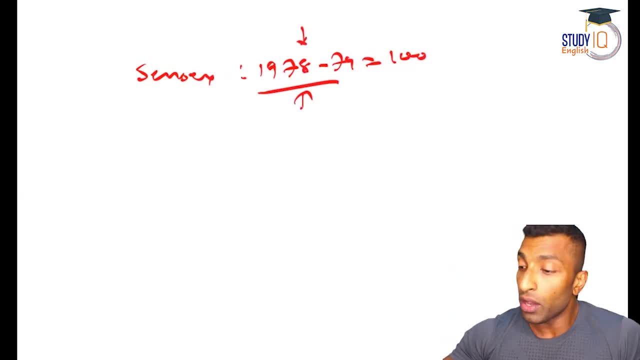 Now it has grown like 50,000, like that. Now, if you suddenly change the base year, what will happen is this 50,000 becomes 100 once again. That is going to be the base value. That will psychologically affect the minds of the people, investors and the markets and everything. 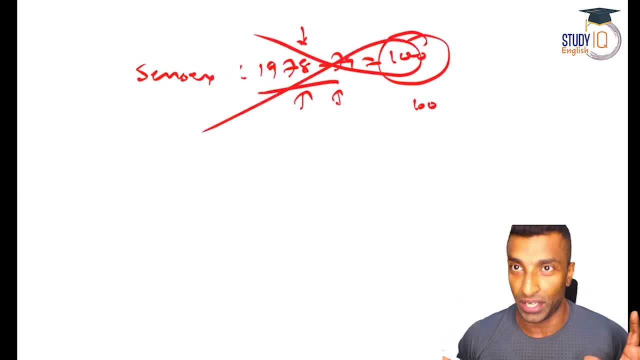 So this Sensex, the base year won't change. It will be like that. I hope this is very clear. Okay, So, based on that, what you can do is you can actually calculate the real GDP. So this is how the calculation is done. 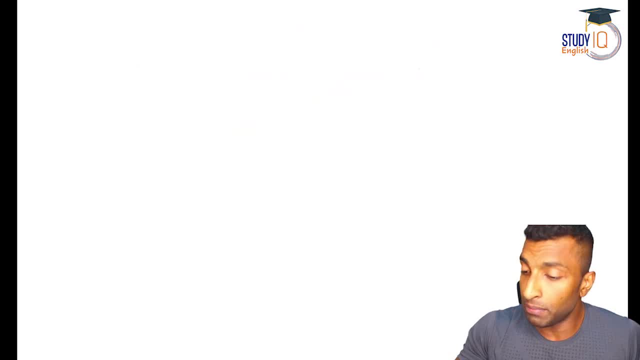 And then, if you see national income, it is nothing but NNP at factor cost. Okay, So this is your national income And then NDP at factor cost. this is going to be your domestic income. So I can take it at current and constant. 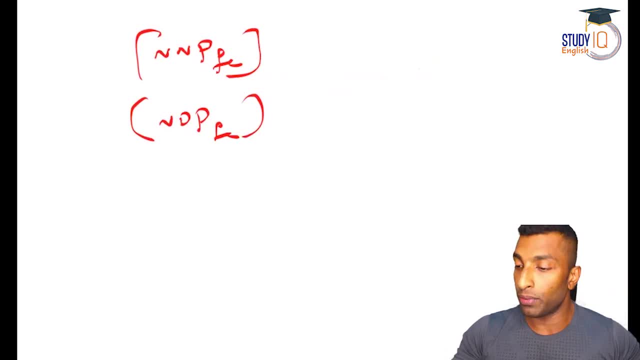 Current is nominal, Constant is real. So if I take it at here, also, constant and current, So this is going to be: current is nominal domestic income. Constant is going to be real domestic income, Similarly the above one also. So in the next session I'll be talking about how this GDP deflator calculation can be done. 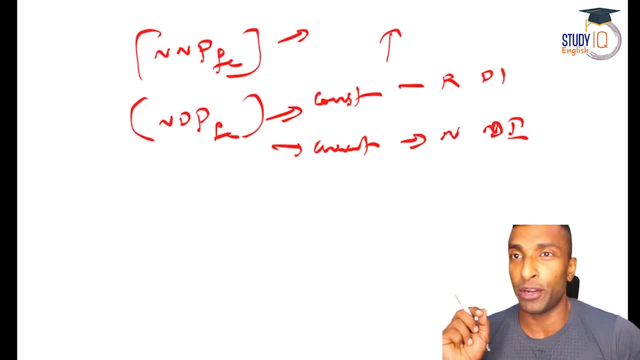 I'll just show one example. At the same time, I'll discuss about the measurement of national income, the methods in which it is measured. Okay, So guys, so far you have watched the video means I'm expecting that you like the video. 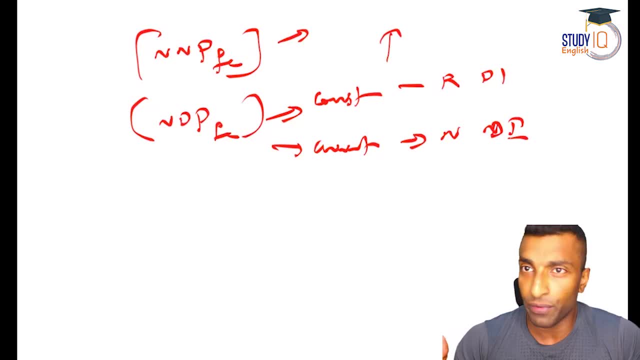 Give me a thumbs up if you like the video, And whatever doubts you have, you can leave a comment. Thank you, Bye, Bye, Bye, Bye. You can comment below and subscribe the channel also. guys, See you in the next video.